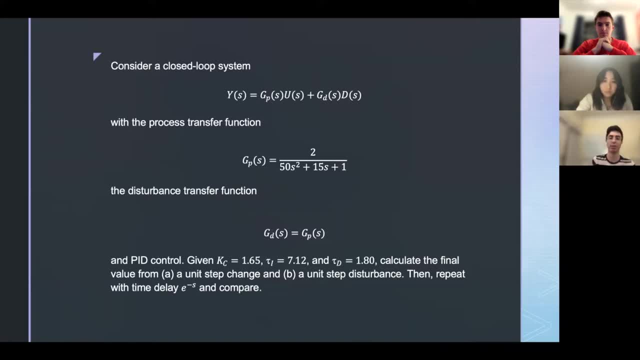 With the process transfer function, gp of s is equal to 2 over 50s squared plus 15s plus 1.. The disturbance transfer function is shown at the bottom of the page and the PID control parameters are given as well, So the goal is to calculate the final value. 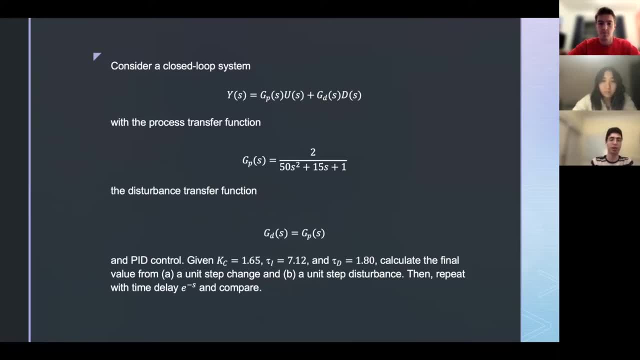 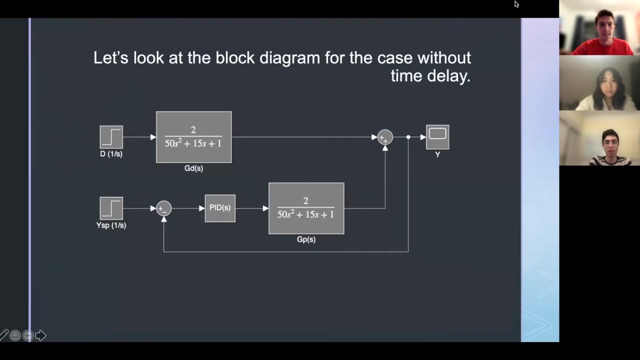 from a- a unit step change, and b- a unit step disturbance. Then we're going to repeat that and incorporate the time delay e to the negative s and compare. So first, before we begin, let's take a look at the block diagram for the case without the time. 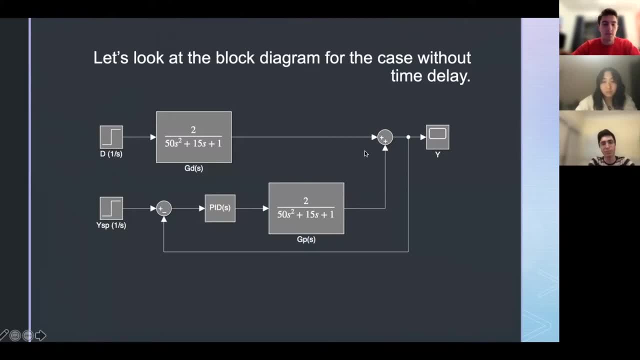 delay On this upper line. here you can see how we have our disturbance function, which in this case is a unit step, so that in the Laplace domain is 1 over s. That disturbance is fed into the disturbance transfer function, which in this scenario is equivalent to the process transfer function. 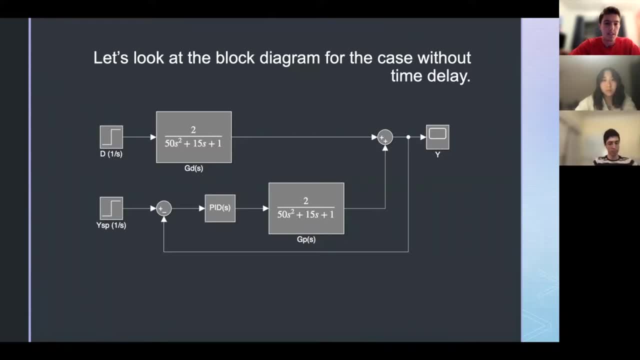 On the bottom. here we have our set point, which again is a unit step. so the Laplace domain makes it 1 over s And here is where we have our feedback loop. So, to begin, YSP will go through, it will go through the PID controller. 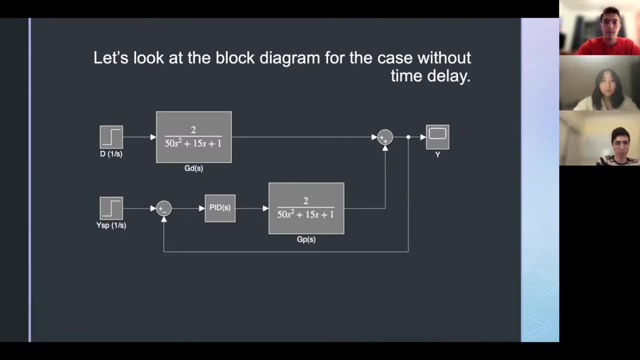 through the process transfer function. That will be added to the disturbance times, the disturbance transfer function, And as that is being output, whatever that value is will be sent back through the system to help correct for any disturbances or general errors that occur along the process. For this first case, we're going to be looking at only when there is a step. 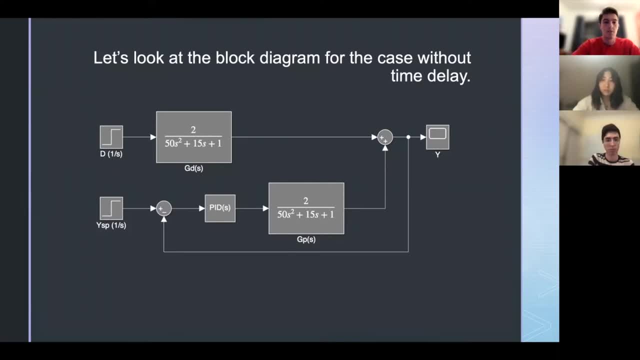 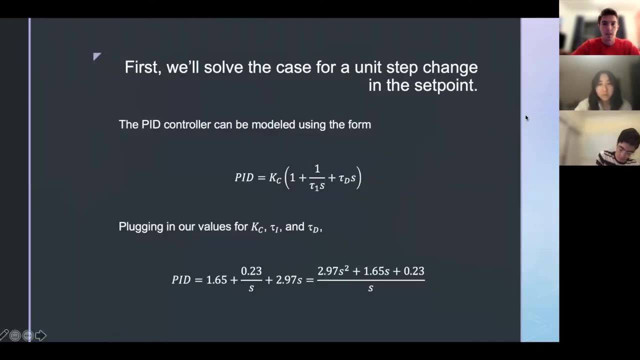 change in the setpoint. so we're going to say that d is equal to zero and that will simplify things somewhat. So, like I said first, we're going to solve the case for a unit step change in the setpoint. So you saw that we had a PID controller and that can be used. that can be modeled using. 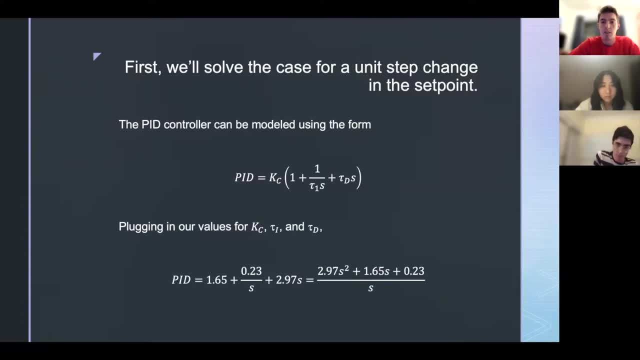 the form PID is equal to Kc times 1 plus 1 over tau 1 times s plus tau d times s. Since they gave us our values for Kc, tau 1, and tau d, we can plug those in and simplify and we are left with PID. 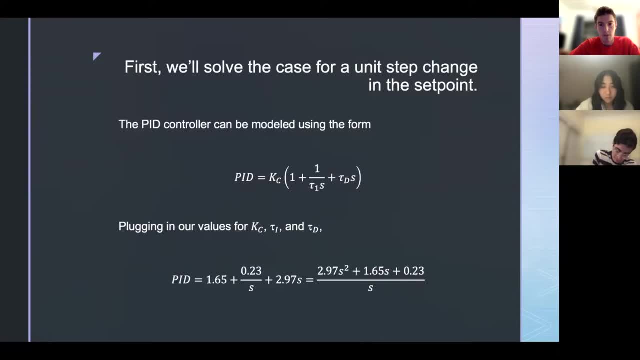 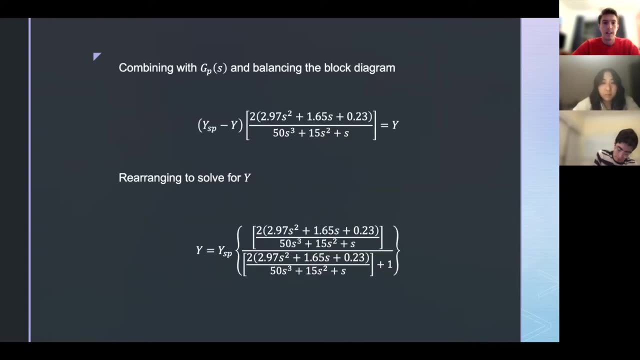 is equal to 2.97 s squared plus 1.65 s plus 0.23 over s. Now we can look back at this diagram. we can combine PID control with Gp of s and then balance the block diagram. What we mean by balancing the block? 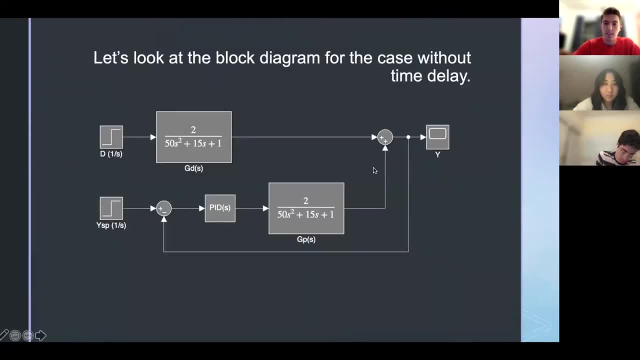 diagram is. we're going to look at all these junctions here. So since the disturbance is zero, we're basically going to treat this as just a straight line into the scope, leaving our only junction as this junction right here. So if we look at what we have going in, we have ysp minus y. 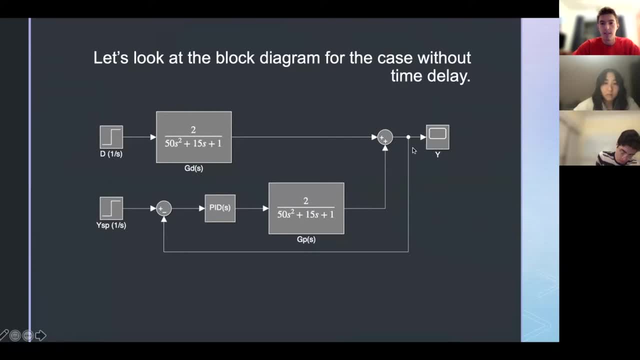 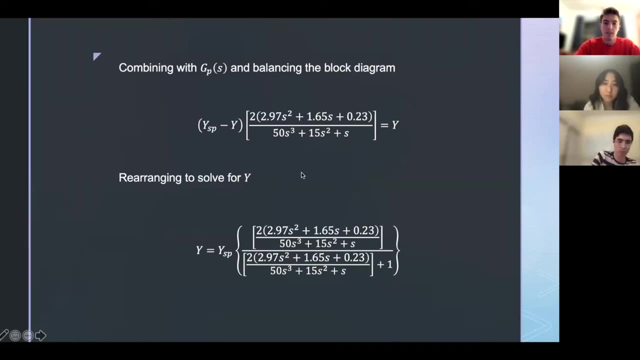 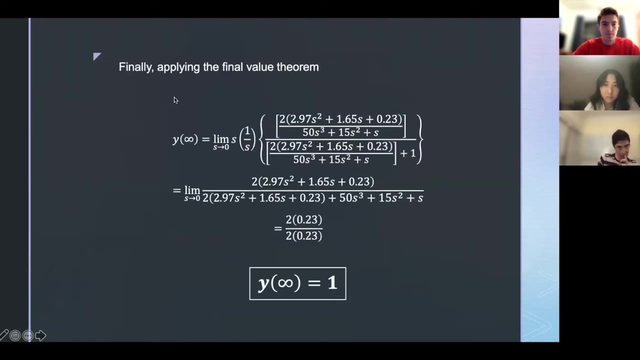 times PID times Gp of s is equal to y, So of course we can rearrange to solve for y. We're left with this kind of nasty equation on the bottom, but I promise it will simplify very easily. Since we have this equation, we're going to apply the final value theorem in order to find: 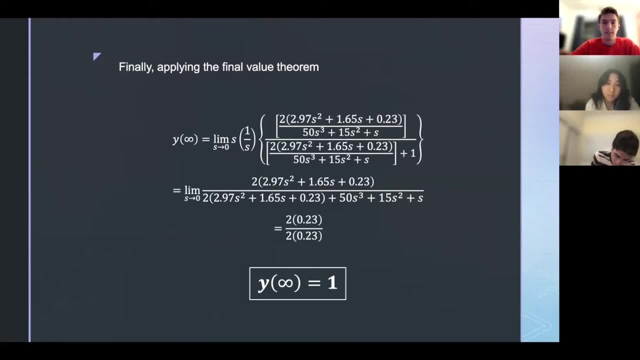 our, our final value, as time goes to infinity. So our step change is 1 over s and when you're using the final value theorem, you do the limit as s goes to 0 of s times, whatever the Laplace domain is times y. As you can see that s times 1 over s cancels out. 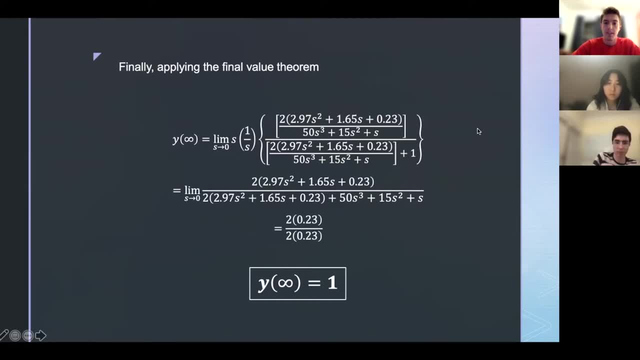 We can simplify this nasty bracket right here and we're left with this long equation Plugging in 0 wherever s is. we are left with 2 times 0.23 over 2 times 0.23.. Which of course simplifies to y. when time goes to infinity is equal to 1.. 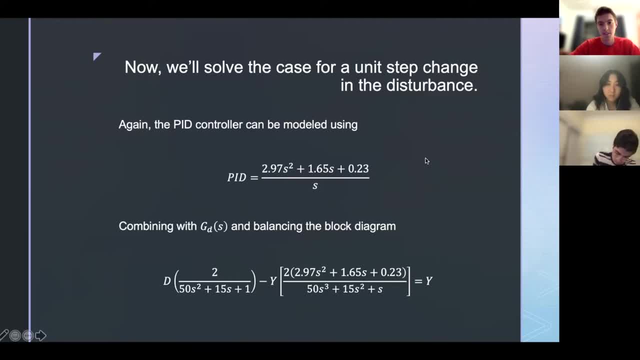 Now that we've done that, we're going to look at the case for unit step change in the disturbance, Just as we we disregarded disturbance in the case that we're looking at the set point. in this case, we're going to disregard the setpoint as we look for disturbance. 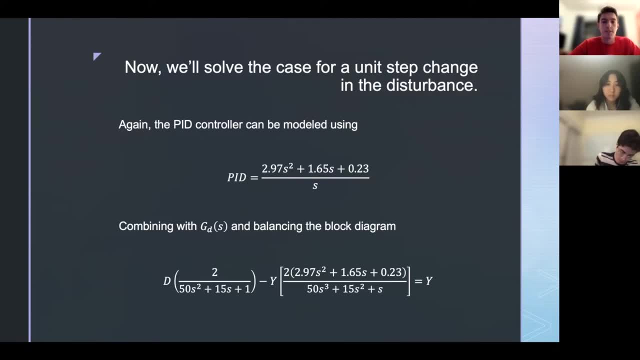 so just to reiterate, our PID controller can be modeled using: PID is equal to 2.97 s squared plus 1.65 s plus 0.23 all over s. Again, combining our disturbance transfer function and balancing the block diagram, we are left with this equation. here Rearranging to solve for y once again. 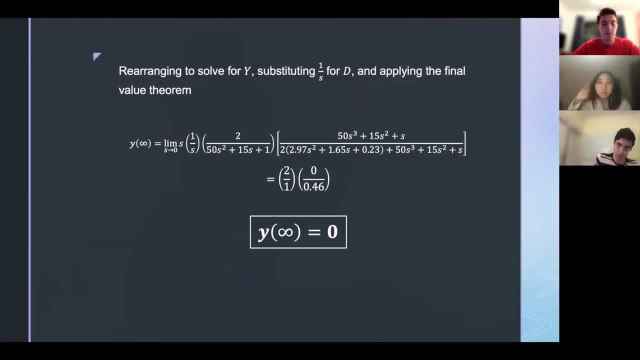 substituting 1 over s for d as the unit step change is 1 over s in the Laplace domain, and applying the final value theorem, we are left with this lengthy limit down below. Thankfully, once again, the s times 1 over s cancels out, and then we can plug in 0 wherever we see an s remaining. 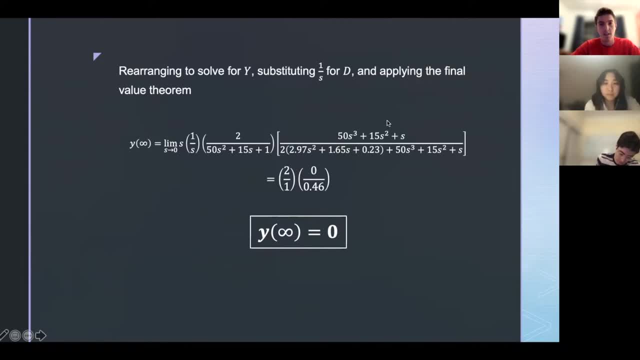 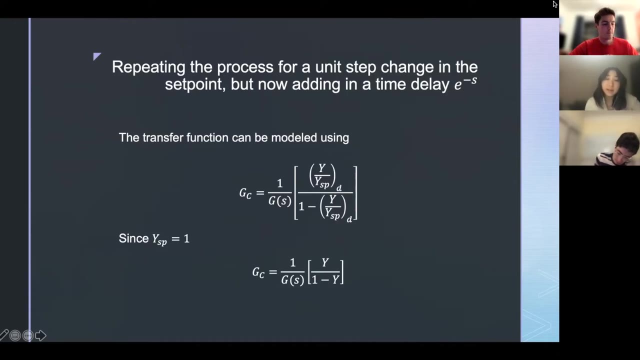 We're left with 2 over 1 simplifies to 2 times 0 over 0.46, which of course means that the final value, as time goes to infinity, is 0.. Now we're going to repeat the process, but this time we're going to add in a unit step change with a time delay. 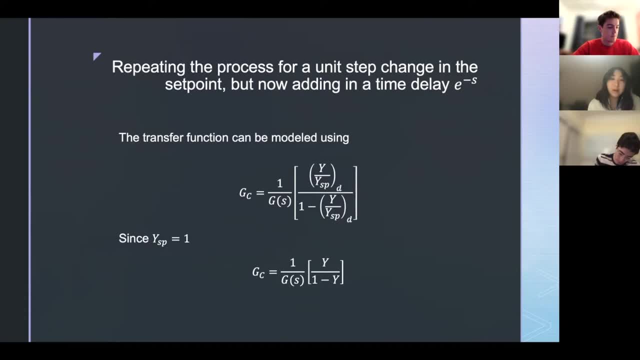 So we can model the transfer function using: gc is equal to 1 over g of s, which is our given transfer function times. y over y set point. with regards to the delay or the disturb: yeah, the delay over 1 minus y over ysp. with the delay, And since ysp is equal to 1, which was given to us, we can simplify this. 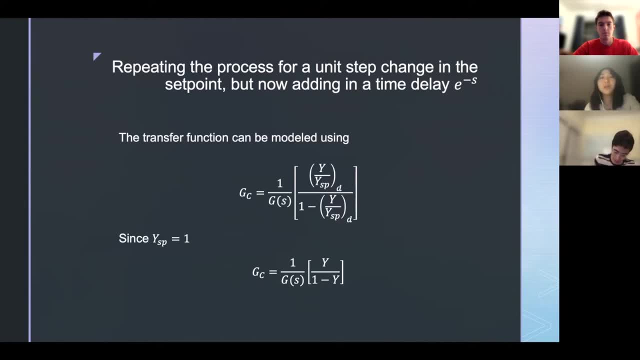 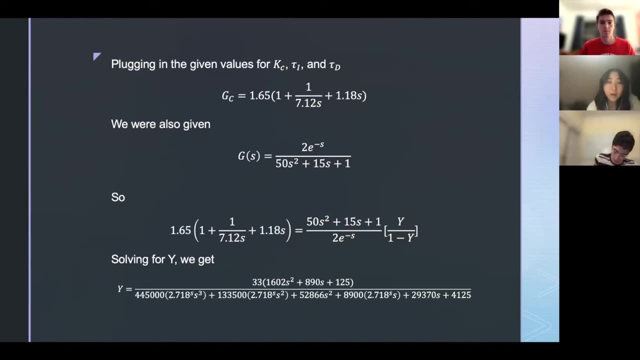 equation slightly to gc is equal to 1 over g of s times y over 1 minus y, And we're gonna plug in the given values from the problem statement to get our gc equation, which is 1.65 times 1 plus 1 over 7.12 s plus 1.18 s. 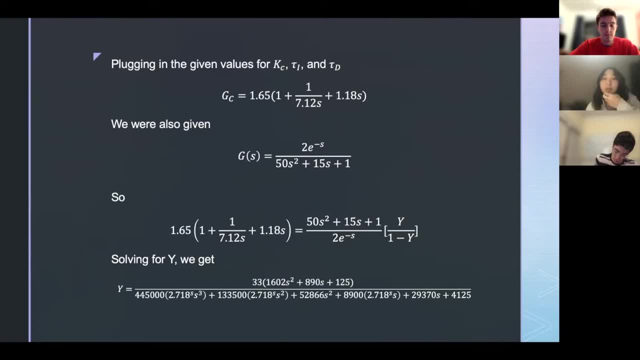 And in the problem statement we are also given our g of s equation, which is 2 times e to the negative s over 50 s squared, plus 15 s plus 1.. And plugging both of these equations into the equation we just derived, we're going to get 1.65 times 1 plus 1 over 7.12 s plus. 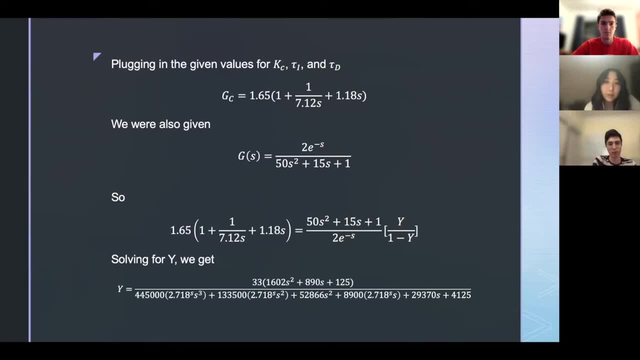 1.18 s, which is our gc, is equal to 1 over our g of s, which is 50 s squared plus 15 s plus 1 over 2 e to the negative s and all of that's times y over 1.. 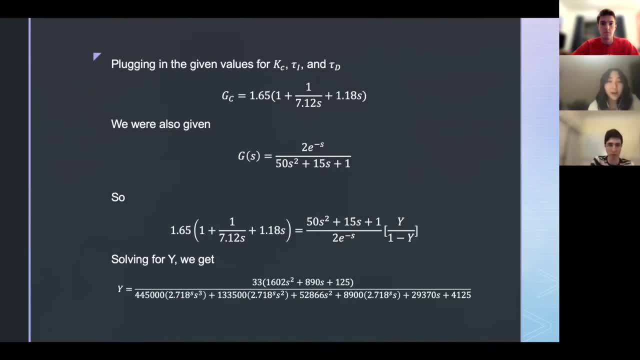 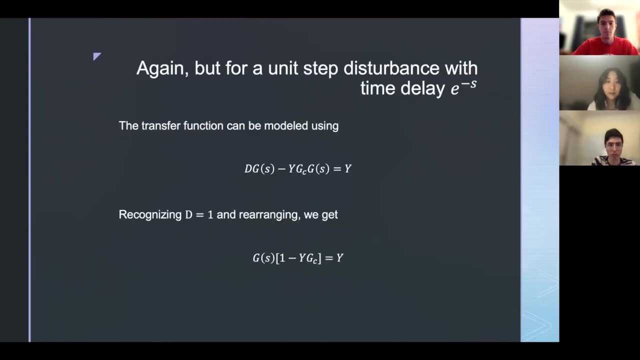 minus y And we use Wolfram alpha to solve for y and we got this huge equation And using the same final value theorem, we're going to take the limit as s goes to 0 of y and when we plug in that big equation for y that we got just now in the numerator, we have left. 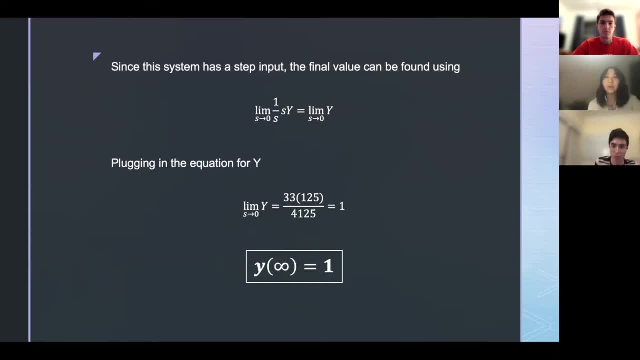 33 times 125, because 125 was the only value that didn't have an s attached to it, as you can see, And in the denominator we have 4, 125.. And when you do 33 times 125 divided by 4125, you get one. 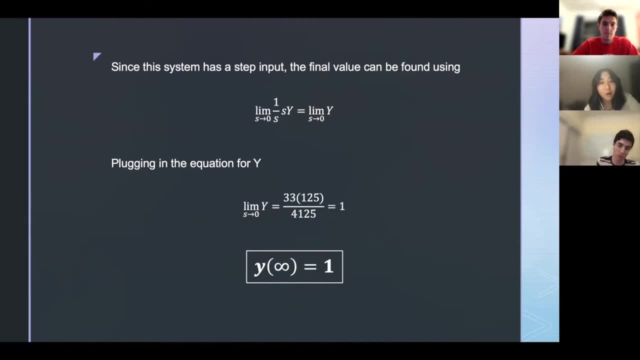 So this indicates that as time goes to infinity, our y value approaches one. We're going to do this, but this time for unit steps. disturbance with time delay, And the transfer function can be modeled using d, which accounts for the disturbance, times g of s, times y minus gc, times g of s, which is equal to y, And since. 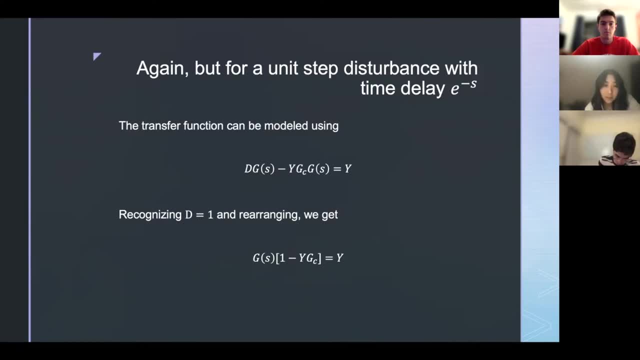 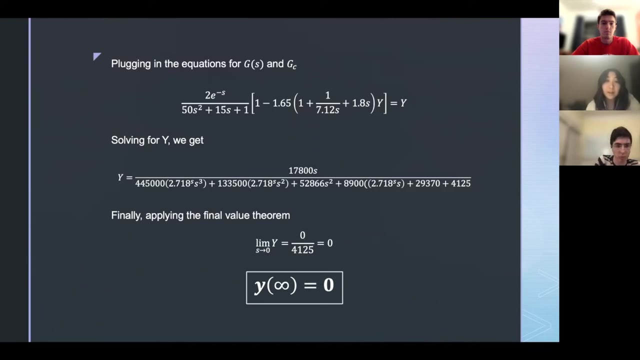 the disturbance is 1, we can plug that in and rearrange the equation above to get g of s times 1 minus y times gc, and that's equal to y. And now we're going to plug in the equations for g of s. 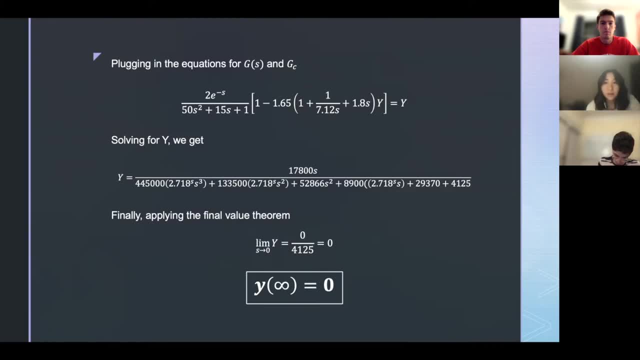 and gc into that equation that we just got, And we can solve for y using Wolfram alpha or a similar online calculator and apply the final value theorem to that, which is as s goes to 0, and, as you can see, the numerator is 17,800 times s, so that'd go to 0.. That's divided by the. 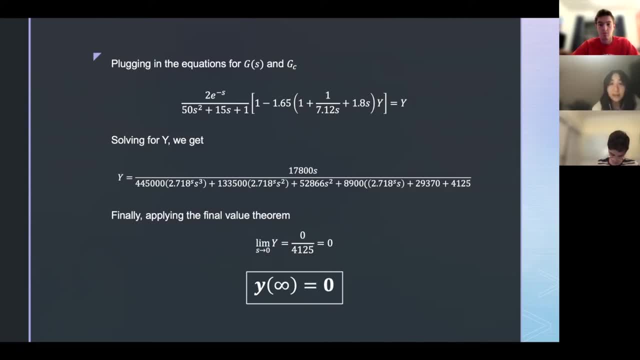 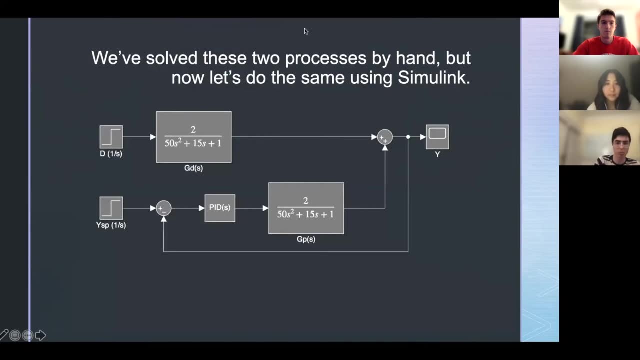 denominator and we get 0. So as time goes to infinity, our y value goes to 0.. All right, so I know everybody loves modeling process dynamics by hand and working with these grueling equations, but now we're going to get into some. 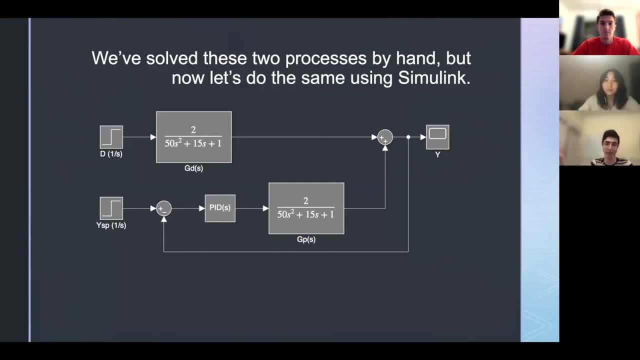 stuff that we're going to talk about. So let's get started simulations to see if we get the same results, because simulations are easier and used in the real world a lot more. But it's important to know the handwriting behind it, so that's why we went. 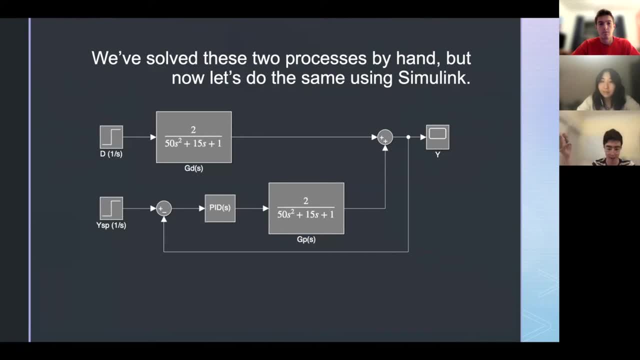 over it so thoroughly. Here is the Bach diagram, which Connor explained so elegantly previously, And the box that looks like your grandparents' television is called the scope, which lets us look at the variable of interest as a function of time after the disturbance was introduced. 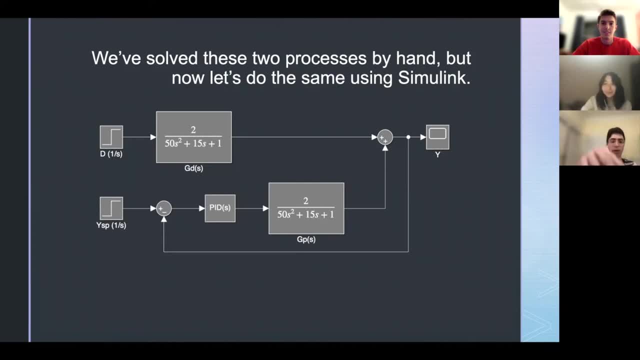 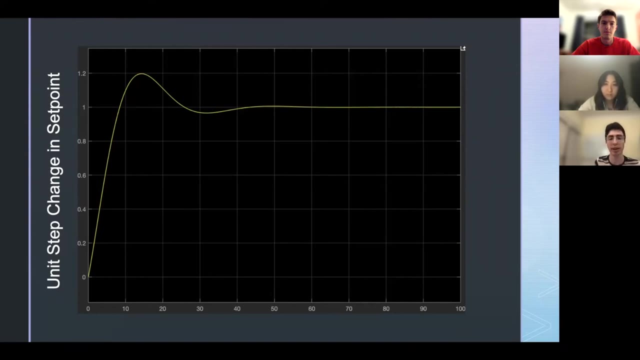 or the change Set point. So we're going to first look at a plot or the scope of a unit step change in the set point and then in the disturbance variable. Here we see the change in set point and it arrives at a steady system response at around 50 time units. it looks like We can just call it seconds or I'll keep it 10 units. So remember that number 50.. 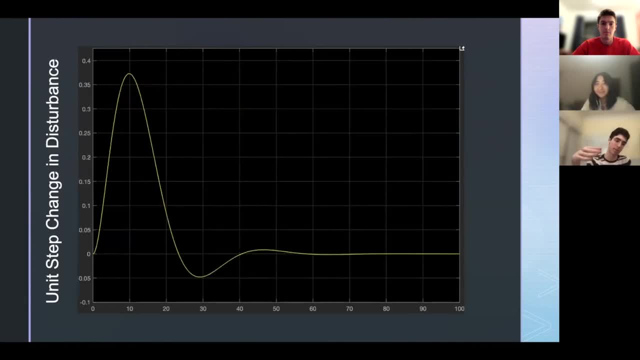 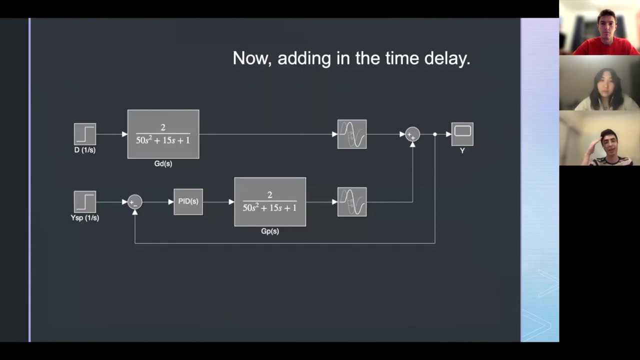 And Next we'll see what happens with the disturbance That also reaches stability at around maybe 60 units. we can call it All right, great, We got 50 and 60 units. Let's see what happens when we introduce a delay. So these these sign boxes, these wavy sort of curves, represent time delay and right now we're working with a time delay of one. so just e to the negative x. 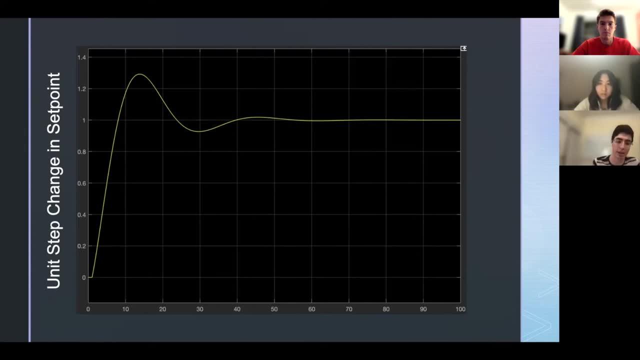 So here the shape looks generally the same And at the start you can see a horizontal shift of one unit And however, the overall stability of the system doesn't reach like entirely. it doesn't become entirely stable until maybe 60 or 70 time units, which is dramatically more than the one unit horizontal shift we had earlier, showing the cascading effect that a time delay can have in the PID loop. 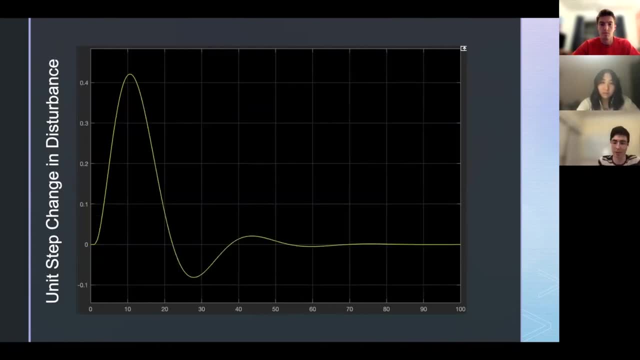 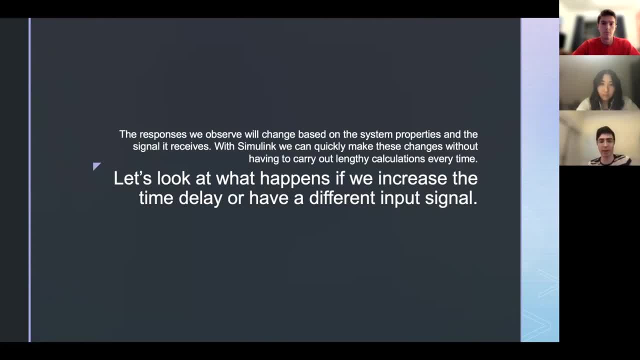 So these responses that we've seen will change based off of the system properties and signals that it receives. Simulink makes these a lot easier so we can explore some more differences in some more and just learn- learn about systems much easier by just plugging in differences in. 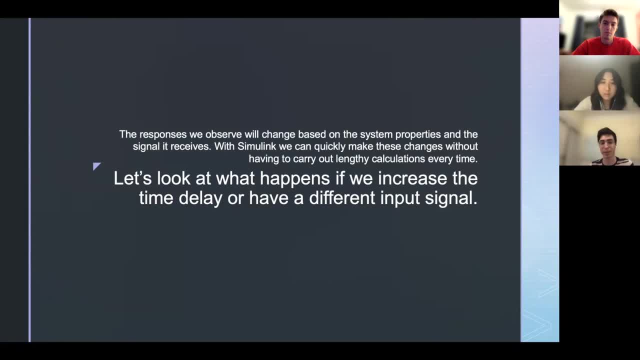 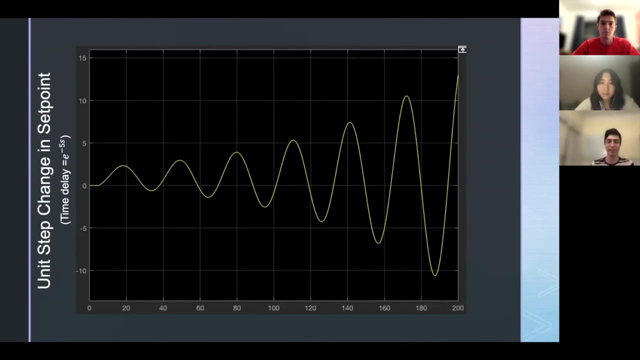 looking at the simulation. Now let's look at what happens if we increase the time delay, and maybe we'll have time to talk about a ramp function too. Now we have a time delay of five e to the negative five s and look, this is not stable, not at all. it just gets bigger and bigger and bigger it's. 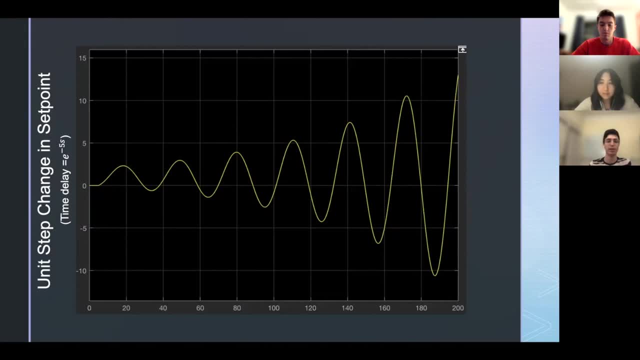 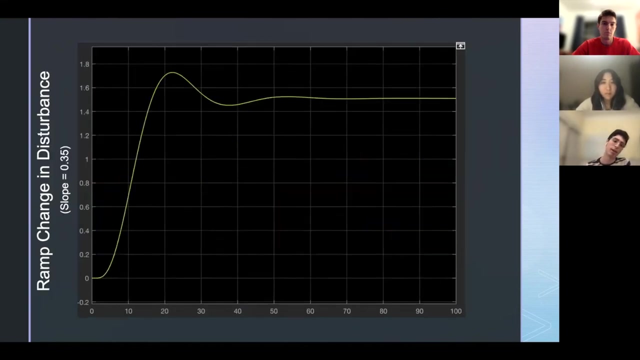 oscillating like crazy. you would want to avoid this. so, in reality, we would be sure to find what type of time delay would result in stability, in instability, and stay well below that. And we included this last plot. this is what happens when the ramp, when there's a ramp, change. 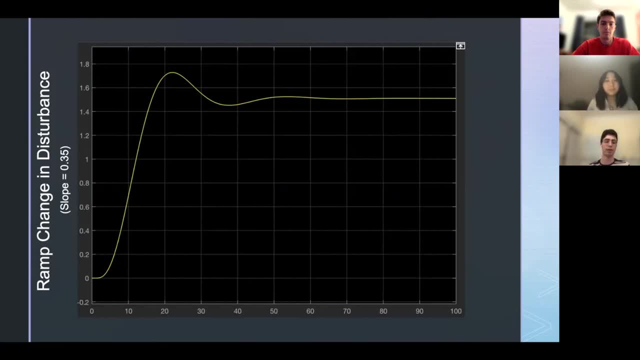 introduced to the dis as a disturbance. we messed around with the slope. we got it to. we said 0.35 because this made the plot look remarkably similar to the unit step. change in set point might be a coincidence, It might not, but we found it interesting. the only difference was that it found stability. 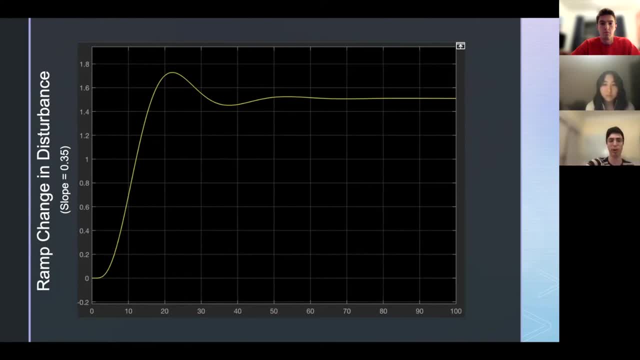 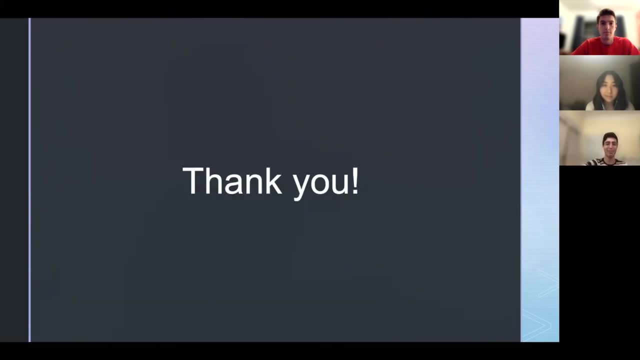 a little bit higher. the stability of the set point was found at one, but this is about 1.5.. Thank you, and thank you for your time. this was very fun. We hope to see you next time. Like and subscribe. 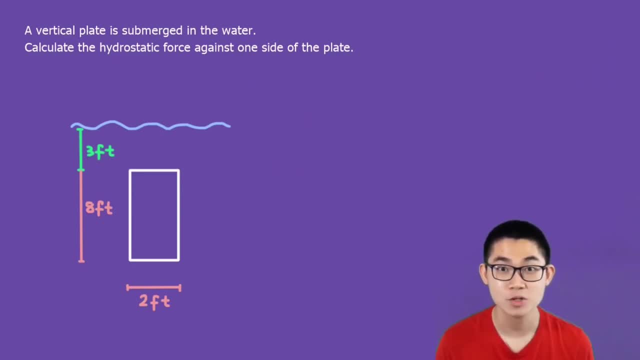 In this video I'm going to show you how to calculate the hydrostatic force on an object submerged underwater. So, for example, here we have a rectangle that is submerged underwater and we have to calculate the hydrostatic force on this object. So, first things first. we know that 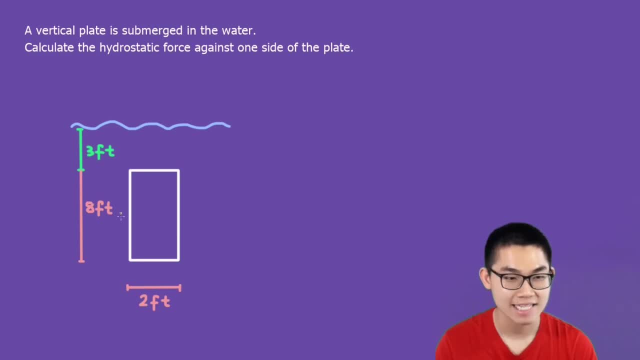 in this rectangle. the width is two feet, the height is eight feet and it's submerged underwater three feet. Let's begin by placing the x and y-axis on this rectangle. So I place the x-axis at the base of this rectangle and you can see that the positive direction is to the right. 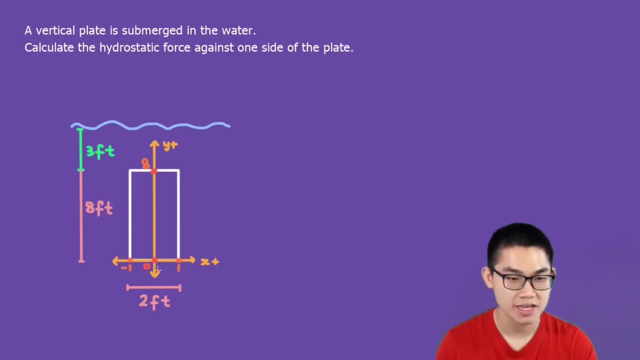 and for the y-axis, I placed it in the middle of the object and the positive direction is upwards. So this point is eight, because we know that the height is eight. so starting at here, at the center, is zero and here is going to be eight. The width is two feet, so the distance from here to here is